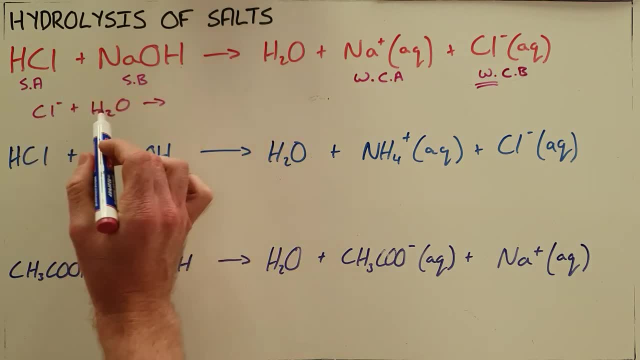 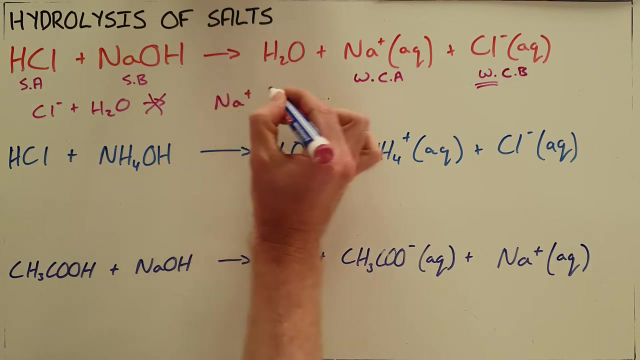 take a hydrogen ion away from a water molecule. so we can therefore say that there is no hydrolysis between chlorine and water, or no hydrolysis reaction. In the same way for sodium we can see that sodium, being a weak acid, does not have a proton to donate to the water. 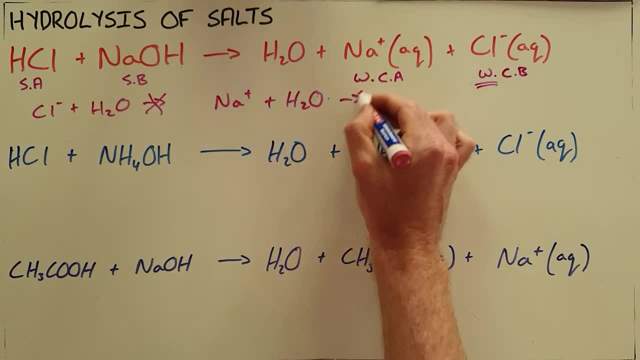 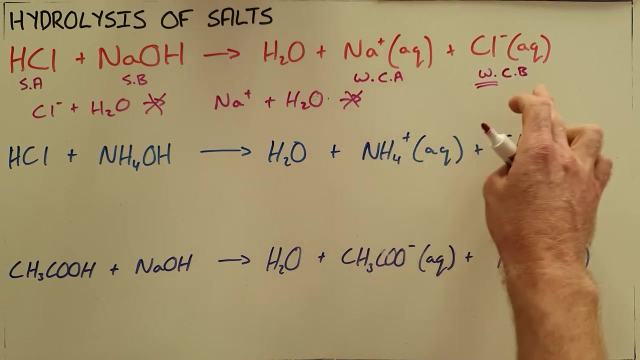 and therefore cannot donate or hydrolyze with the water. so since there is no hydrolysis reaction with the water, there is no further product formed. We'll see what exactly we would expect to form in the next two examples, but that is why we can safely say that this is a neutral salt, because 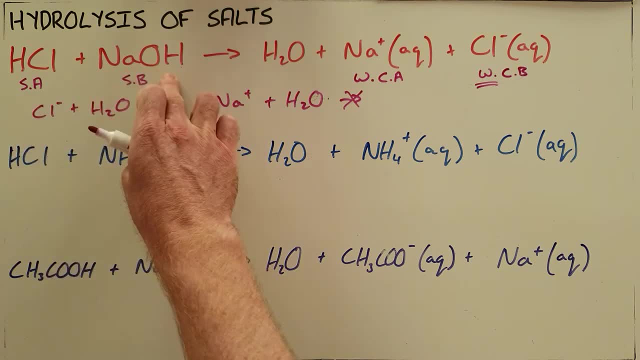 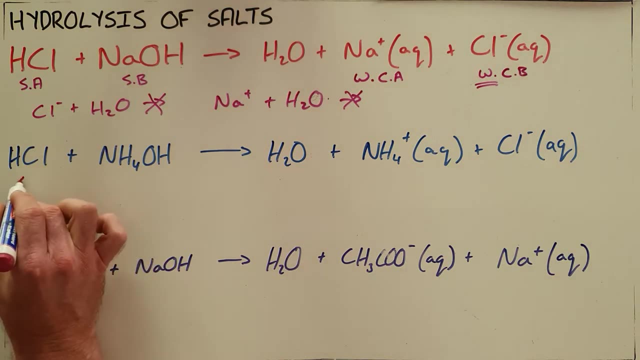 we can see that a strong acid would completely neutralize a strong base and the salt would then be a neutral salt. This is in contrast to a reaction where we have hydrolysis, Hydrochloric acid again, which is our strong acid, and ammonium hydroxide, which we know is a weak 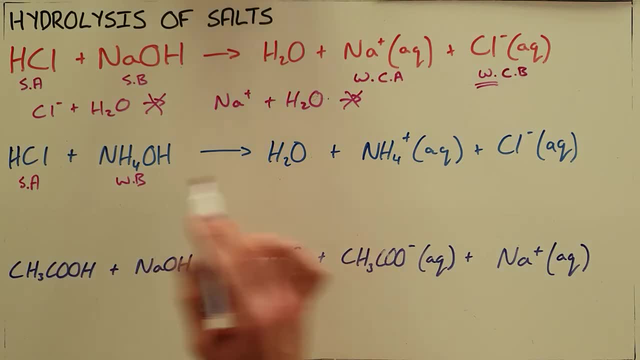 base. Once again it forms water and then the two salts that it forms. the ammonium we can see very clearly is the conjugate acid for this ammonium hydroxide base and since it is a weak base, that must mean that it is a strong conjugate acid. and once again, the chlorine is our weak conjugate base. 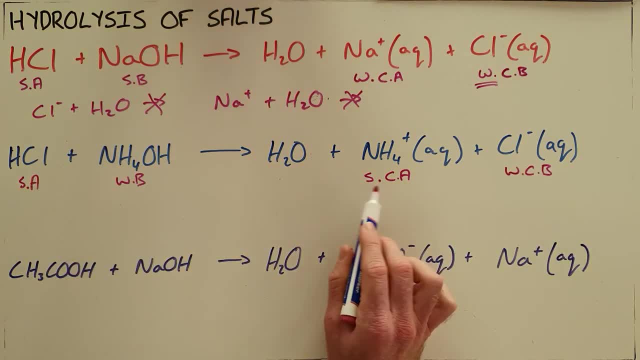 for the hydrochloric acid. So the only new substance here is the ammonium ion, and we are going to see that that ammonium ion undergoes hydrolysis with water because it is a strong conjugate acid, meaning it is capable of donating a proton. and since it can donate, 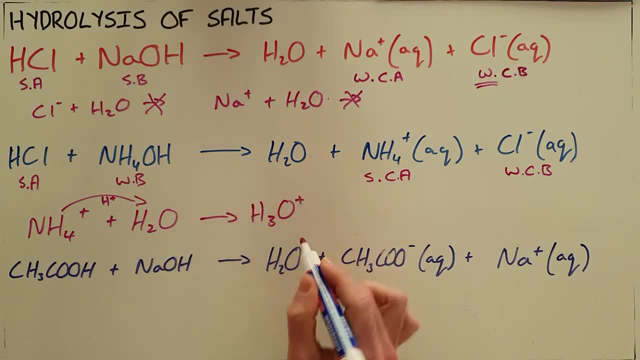 a proton to water, it will form more hydronium ions and obviously some ammonia. but this hydrolysis- the hydrolysis of ammonium with water- clearly shows that our products actually form some ammonium, and what that implies is that, even though we have a neutralization reaction between an acid, 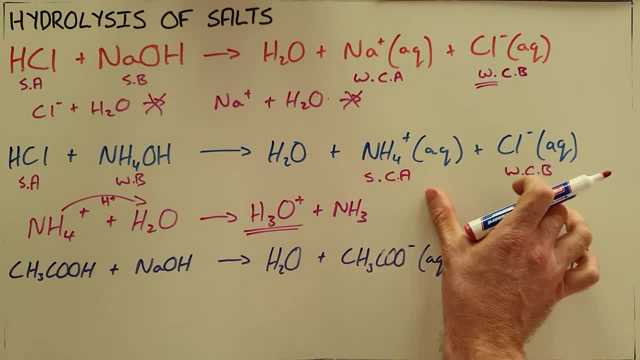 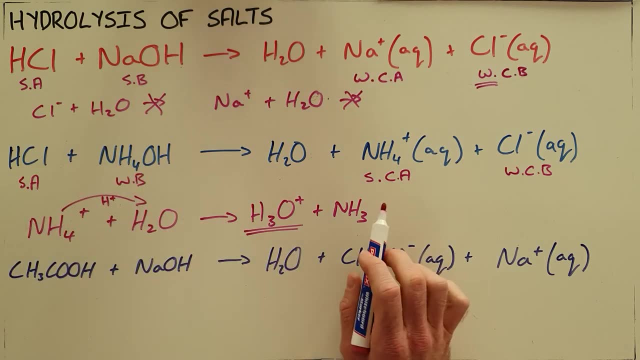 and a base. our salt, the ammonium chloride molecule is still acidic because we had a strong acid and a weak base. So the implication here is fairly standard, in that we would expect that a strong acid plus a water molecule would be a strong conjugate acid.